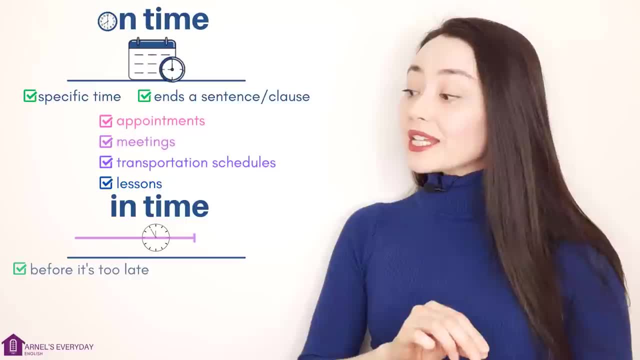 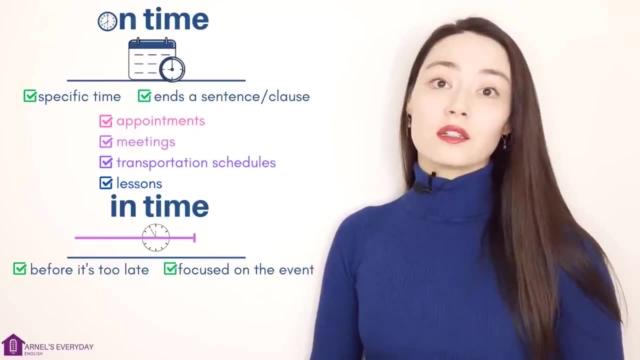 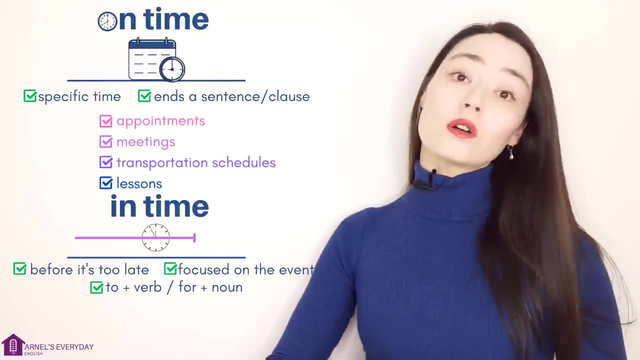 When do we use in time Before? it's too late And we aren't focused on the specific time, we're more focused on the event. Let the grammar help you. We normally say in time two plus verbs or in time four plus noun. I usually work late. 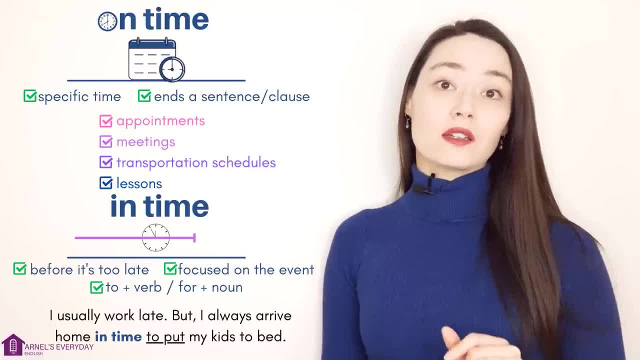 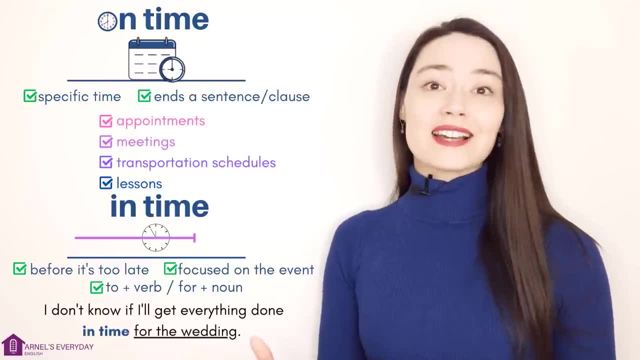 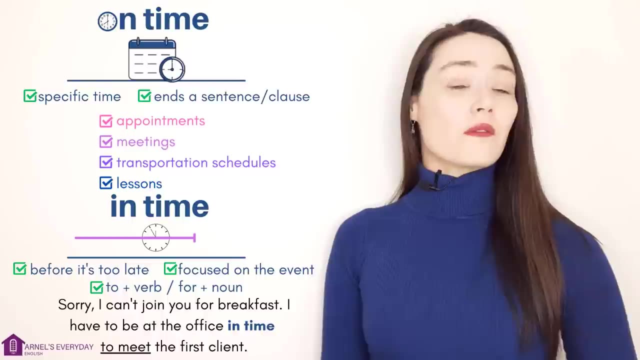 but I always arrive home in time to put my kids to bed before it's too late. I don't know if I'll get everything done in time for the wedding. Sorry, I can't join you for breakfast. I have to be at the office in time to meet the first client. 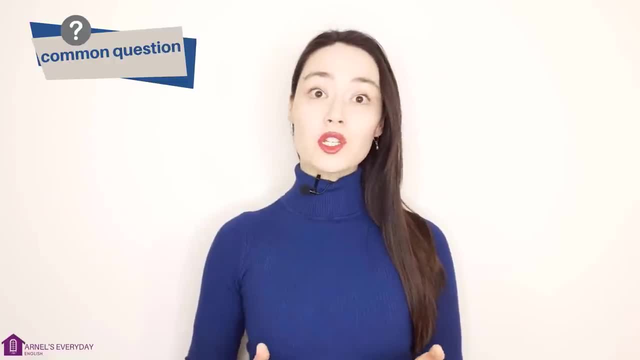 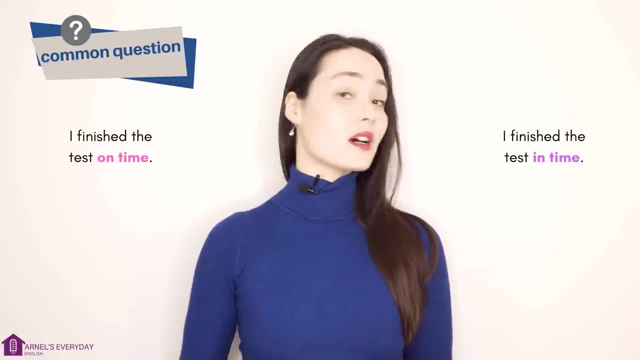 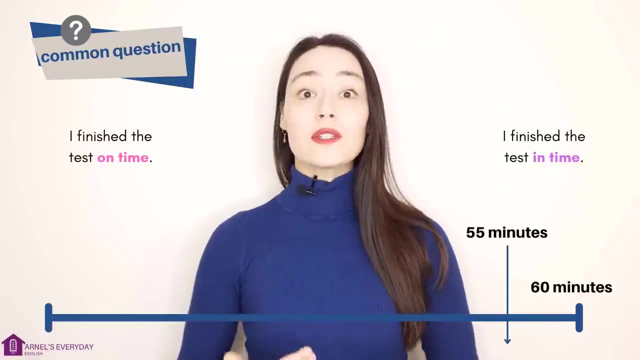 before it's too late. Here's a common question: What's the difference between I finish the test on time and I finish the test in time? Let's say you have 60 minutes to complete a test and you finish in 55 minutes. 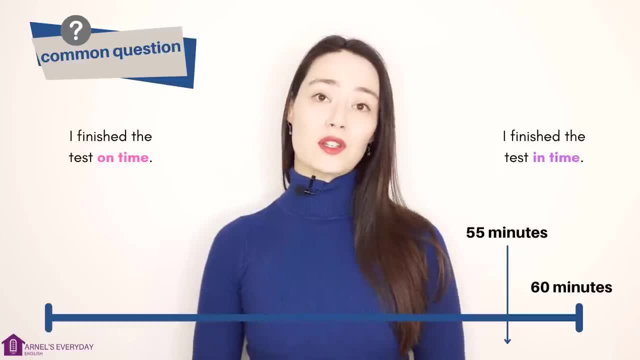 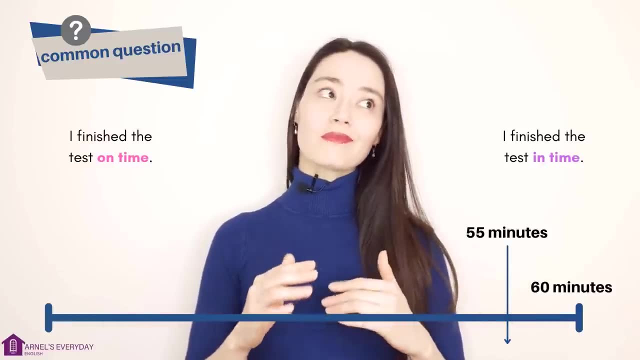 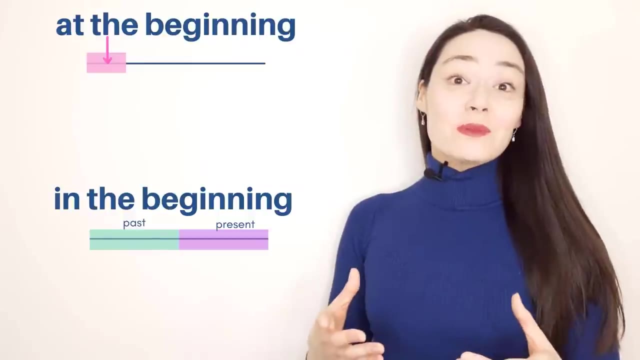 Here. either sentence will give you the same information. There is no difference. But situations where you can use these two phrases interchangeably are not very common. So do remember those differences At the beginning or in the beginning. I have two more lines. 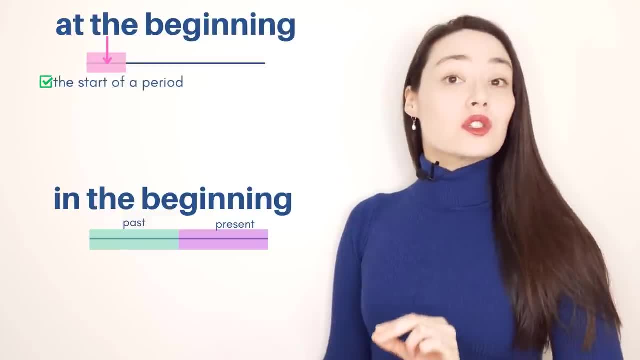 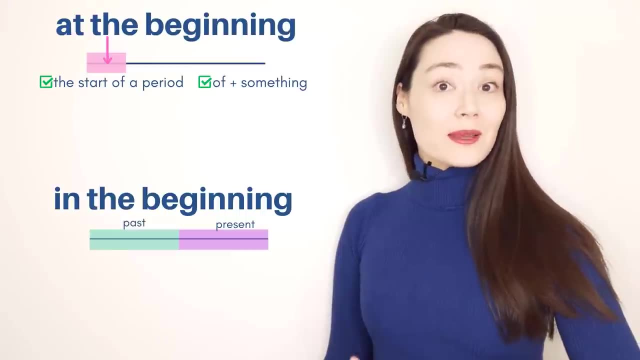 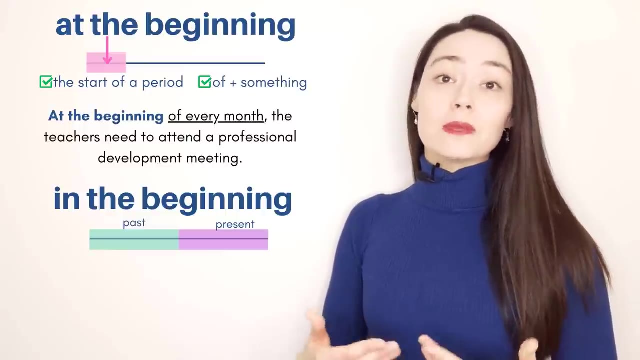 At the beginning. We are focused on the start of a period. Let the grammar help you. We normally say at the beginning of something, At the beginning of every month. the teachers need to attend a professional development meeting At the beginning of every month. this could be. 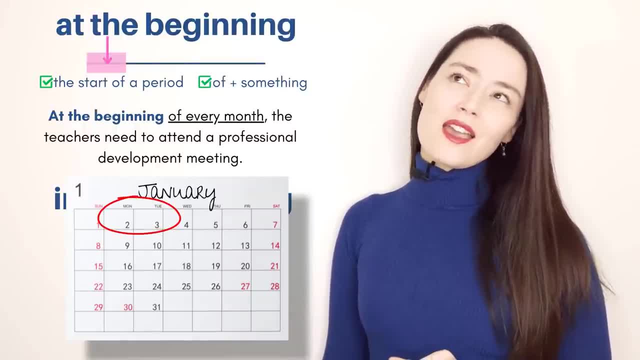 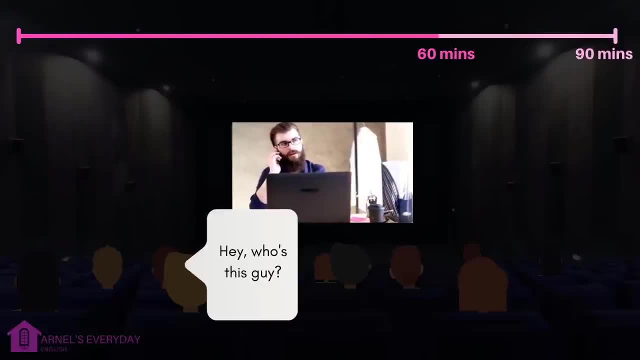 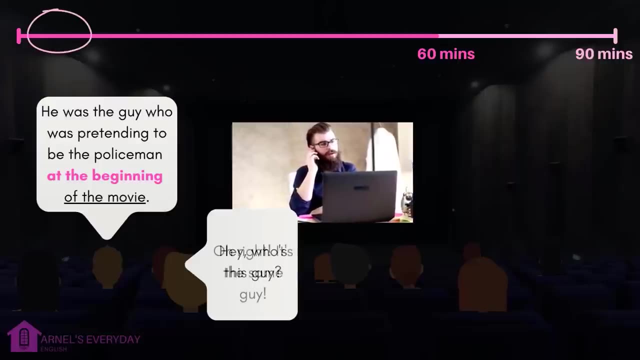 the first Monday or Tuesday of every month. And let's say, a movie is 90 minutes long and we are one hour into the movie. Hey, who is this guy? He was the guy who was pretending to be the policeman at the beginning of the movie. All right, it's the same guy. 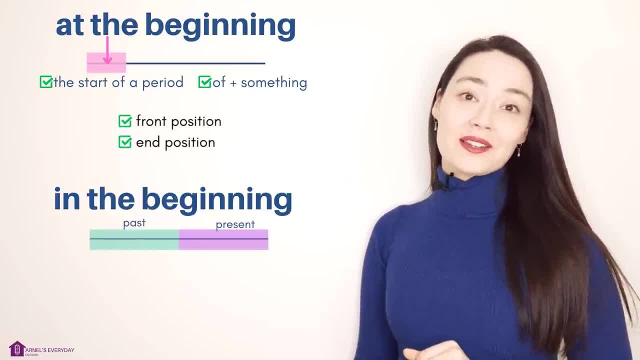 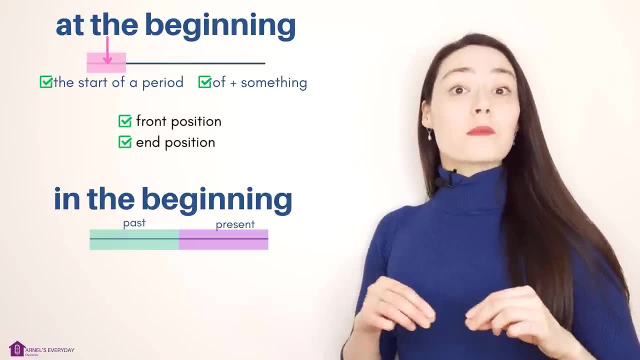 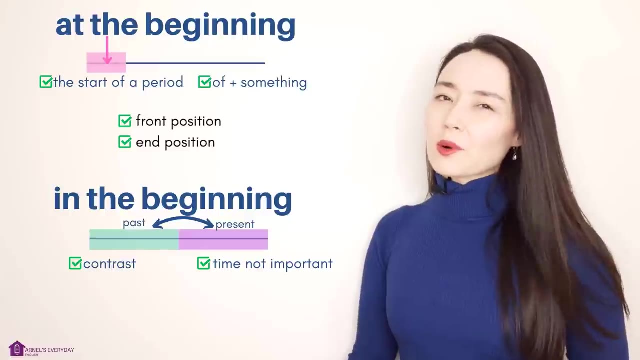 Front position and position. both are fine In the beginning. The start is different from now. There is a contrast And we don't know specifically when. That's not important. I want you to think about in the beginning, like the word originally. 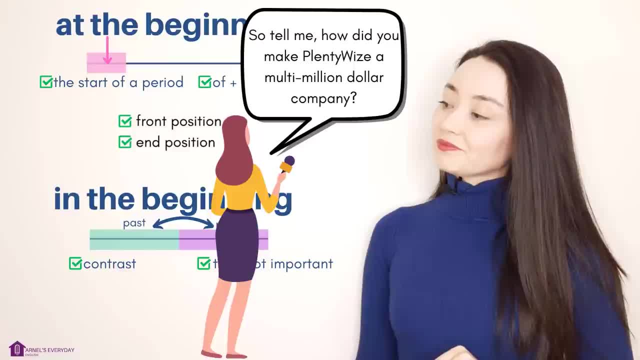 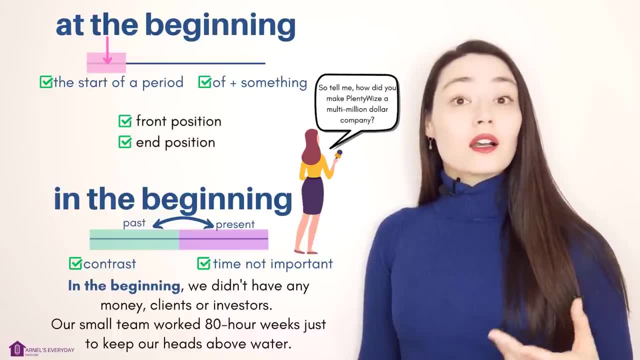 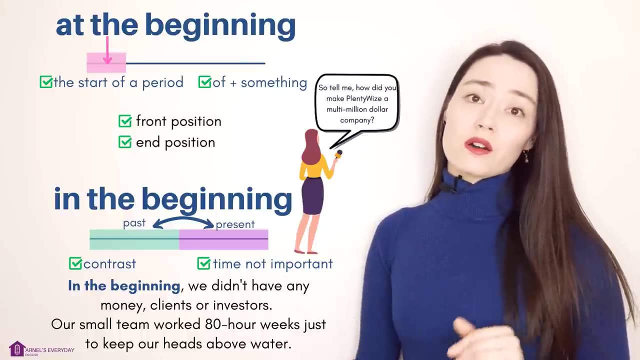 So tell me, how did you make Plentywise a multi-million dollar company? In the beginning we didn't have any money, clients or investors. Our small team worked 80 hour weeks just to keep our heads above water. There is a contrast between the multi-million dollar company now and the company. 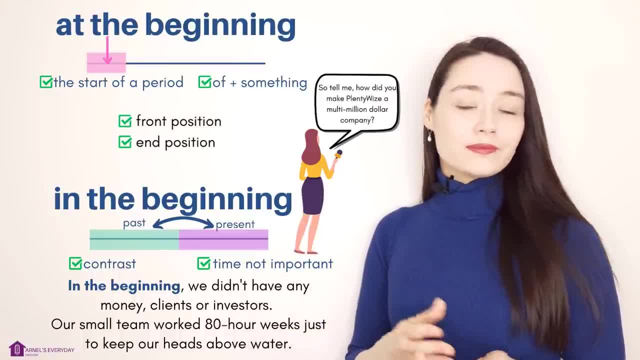 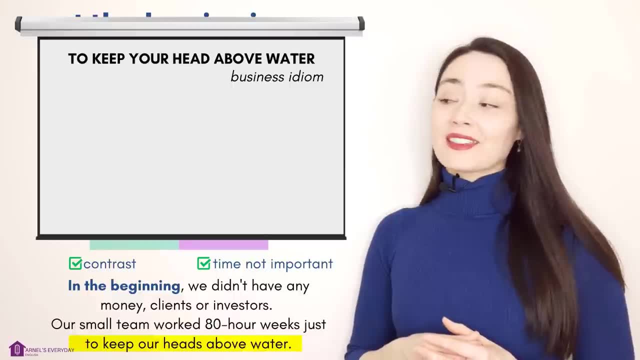 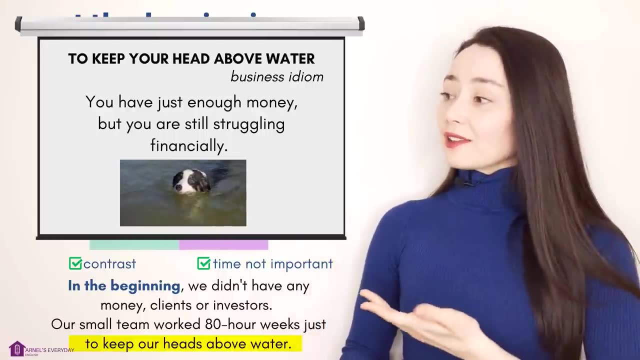 years ago, Do we know specifically when? No, And to keep your head above water is a great business idiom. It means you have just enough money, but you're still struggling financially, Kind of like this dog swimming: Your head is above water, but you're still having difficulties. 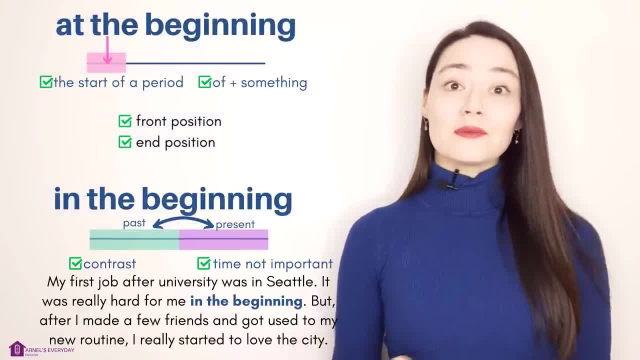 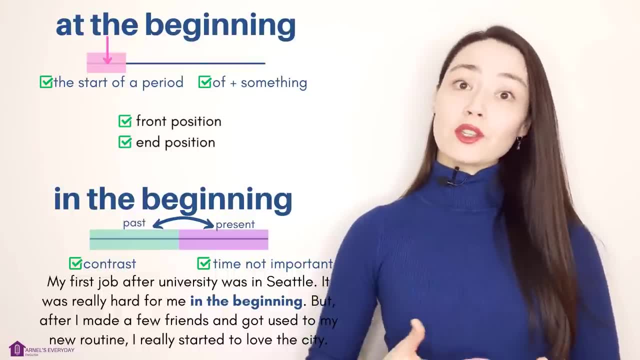 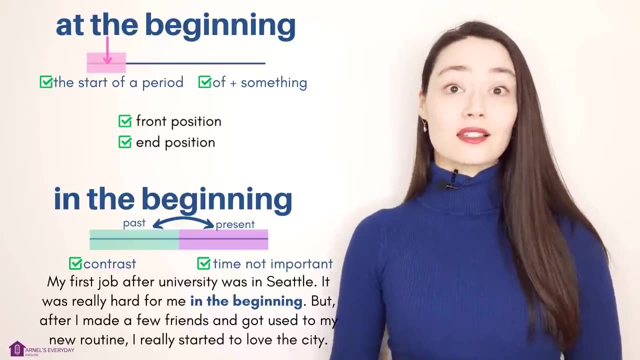 My first job after university was in Seattle. It was really hard for me in the beginning, but after I made a few friends and got used to my new routine I really started to love the city. Is there a contrast? Yes, Do we know specifically when? 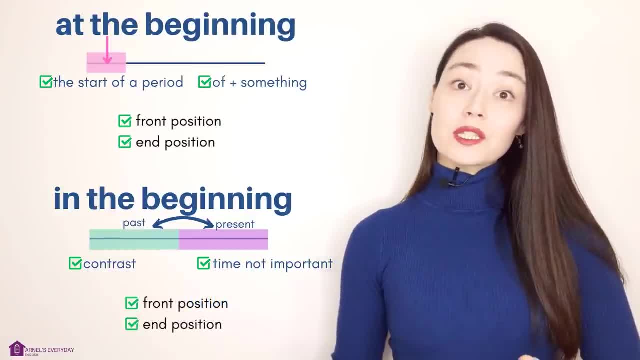 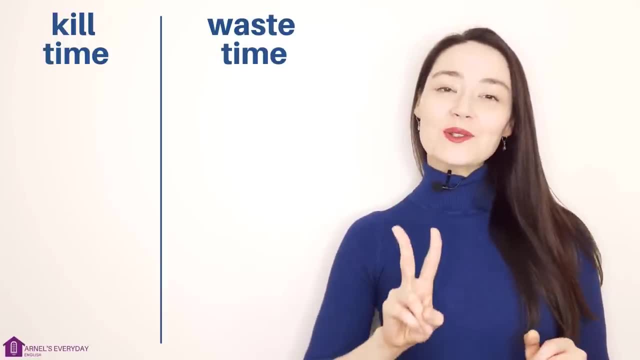 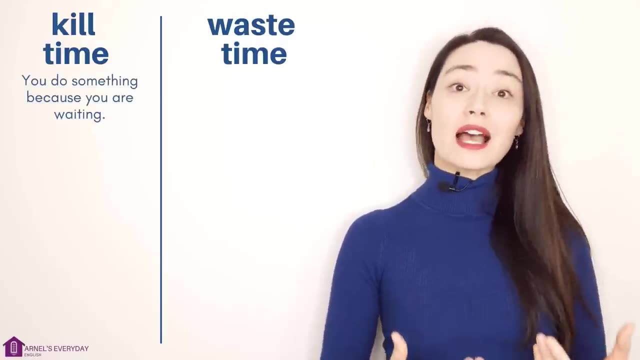 specifically when No. So front position and position- both are fine. Kill time or waste time- These are two really fun phrases. When we kill time, we do something because we're waiting for something else. That waiting part. is really important. When we waste time, it's really like we're throwing time into a 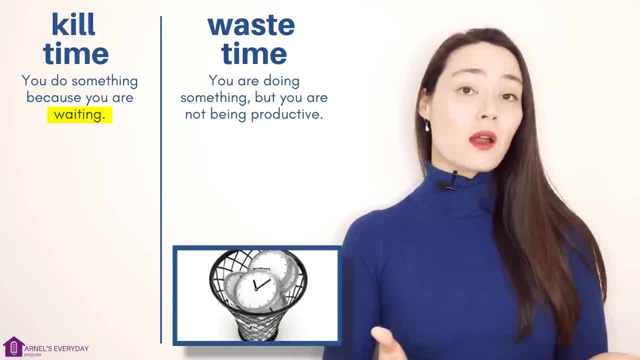 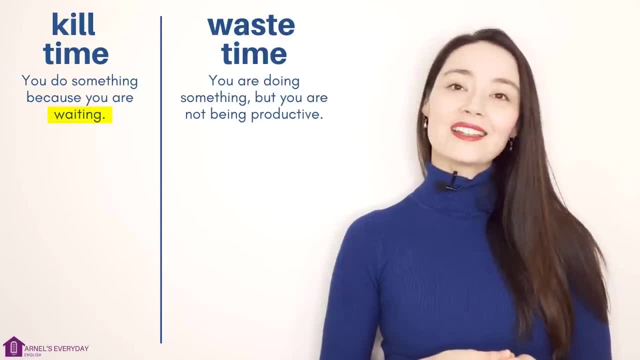 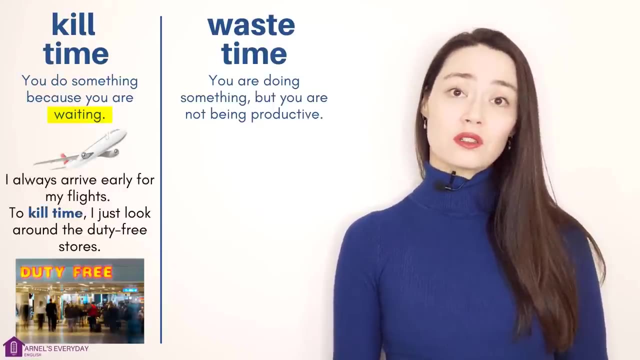 trash can. We're doing something but we're not being productive. We can even say we're being lazy. I always arrive early for my flights. To kill time. I just look around the duty-free stores. We normally have a lot of time to kill at. 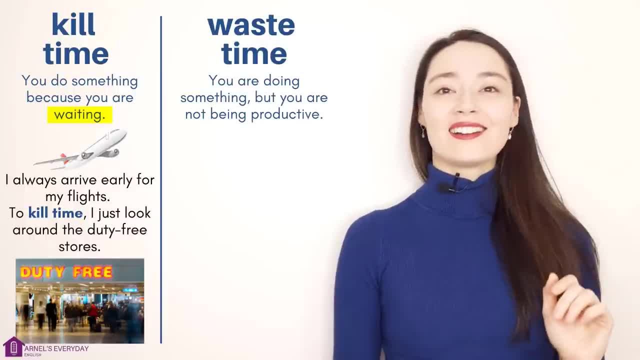 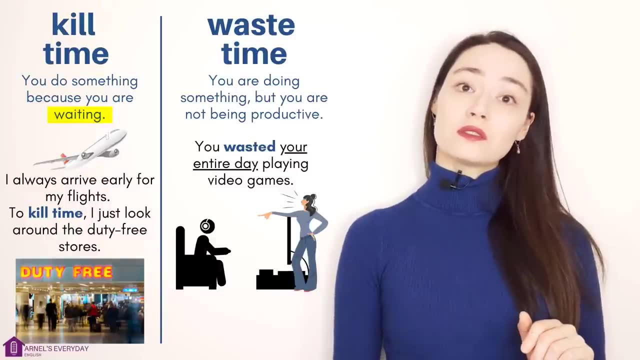 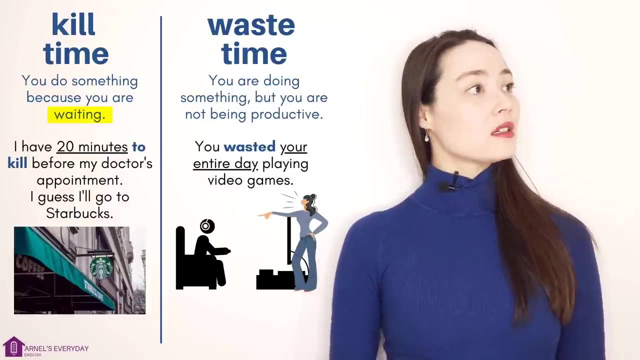 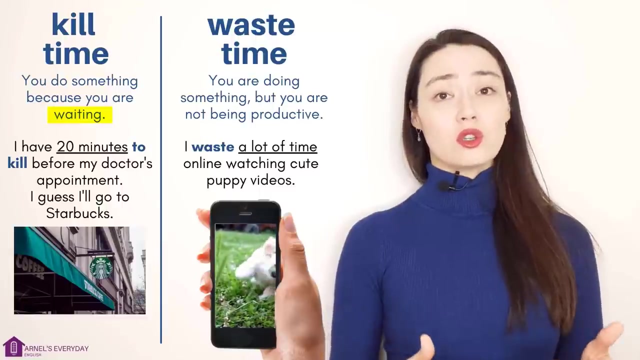 airports, right? Hmm, you wasted your entire day playing video games. I have 20 minutes to kill before my doctor's appointment. I guess I'll go to Starbucks. I waste a lot of time online watching cute puppy videos, And we can. 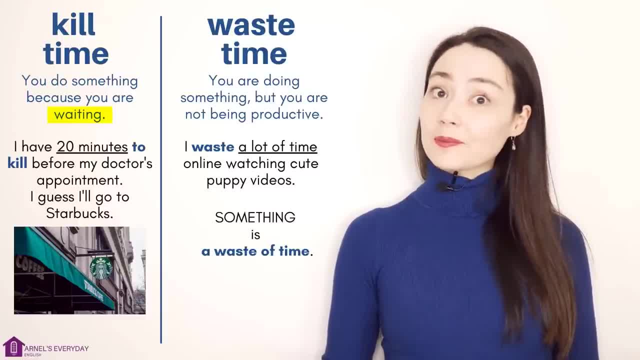 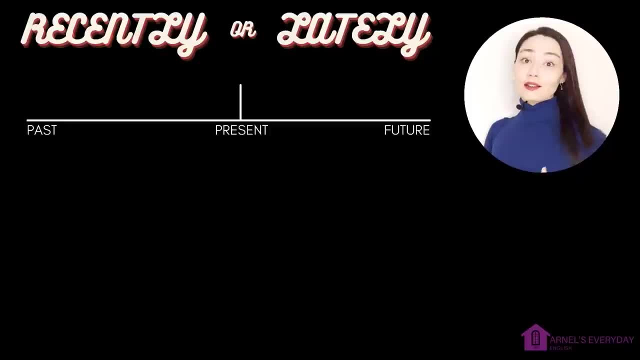 also say something is a waste of time. Ugh, why am I the only one here? This is such a waste of time. Recently or lately- Look at my timeline here I have the past, the present and the future, Both recently and lately. describe this period here, Near the 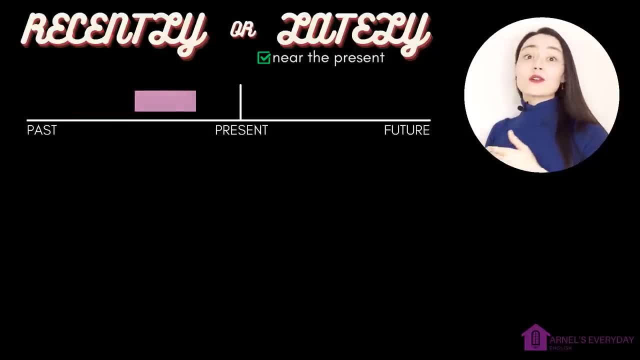 present, Not too far in the past, near the present. Do we know specifically when? No, Will this action or situation continue into the future? Maybe, maybe not. The good news is: normally we like to do things in a certain time palette, As I don't want to be around you. 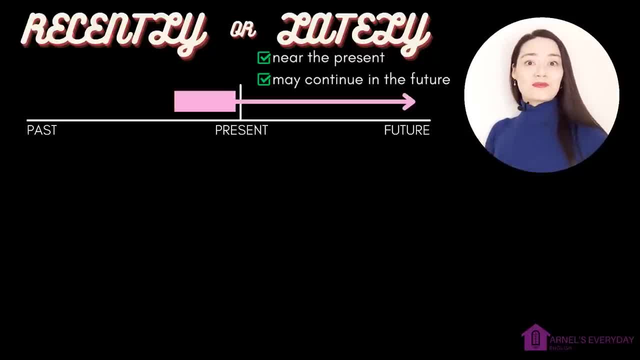 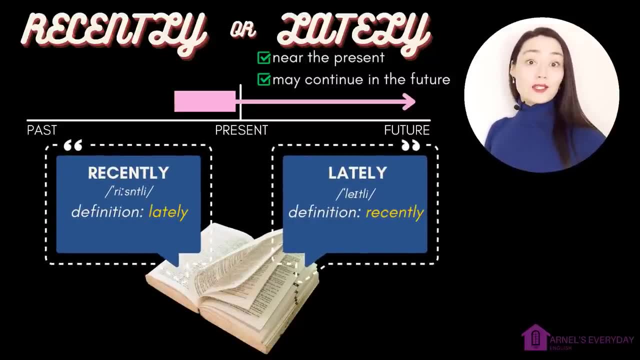 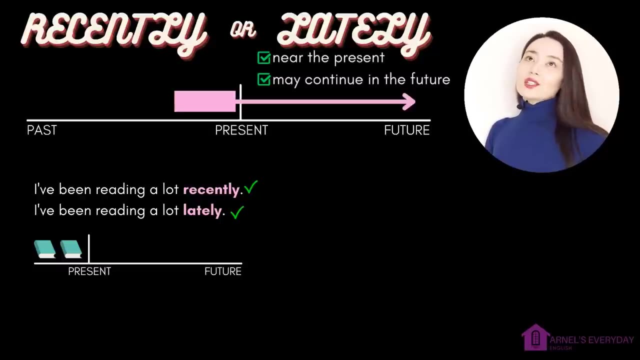 these two adverbs can be used interchangeably. If you look in a dictionary, the definition for recently is lately and the definition for lately is recently. I've been reading a lot recently. I've been reading a lot lately. Maybe I started reading two months ago. It's rained a lot recently. It's rained a. 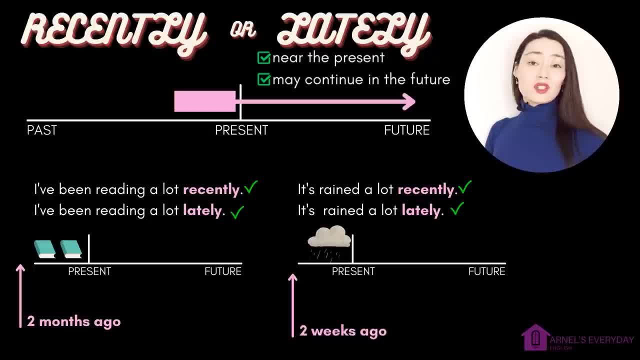 lot lately. Maybe the heavy rain started two weeks ago, something like that. And look at the tenses I'm using: Present, perfect, continuous and present perfect. This is because these actions are close to the present, so we have that past to present connection. Past simple will also be okay if we're describing the recent 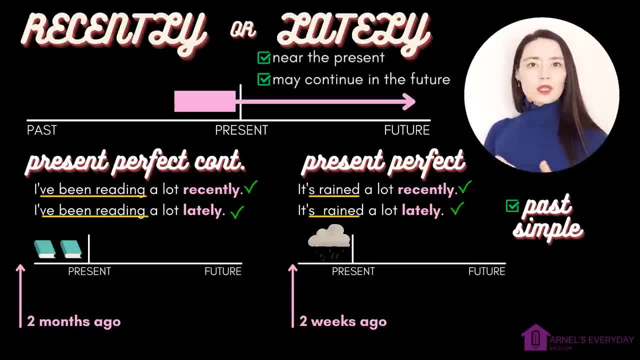 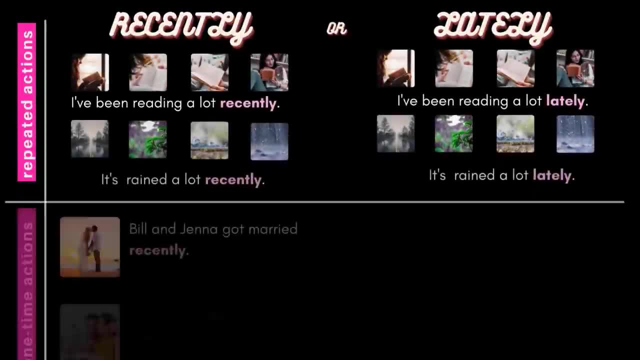 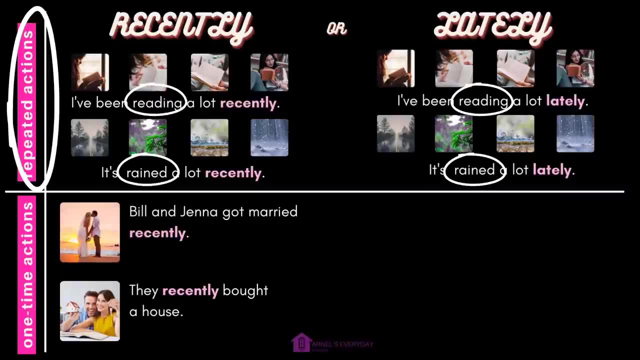 past, But can there be a difference between these two words? Yes, So I've made a little chart for you. We can use lately and recently for repeated actions like reading raining. These are things that can happen multiple times If it's one action. use recently, Bill, and. 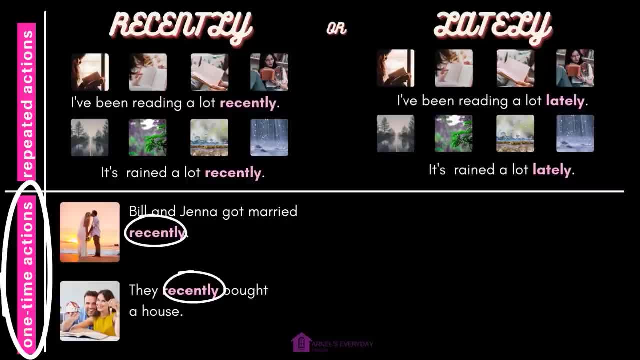 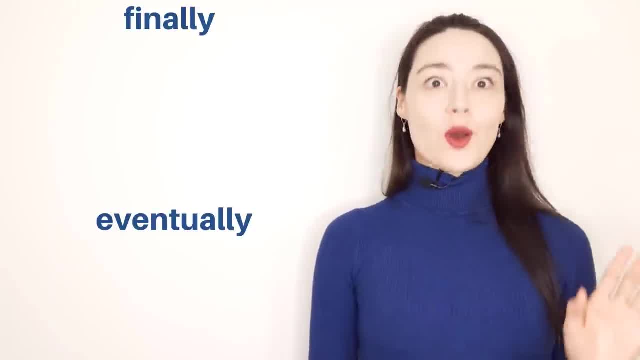 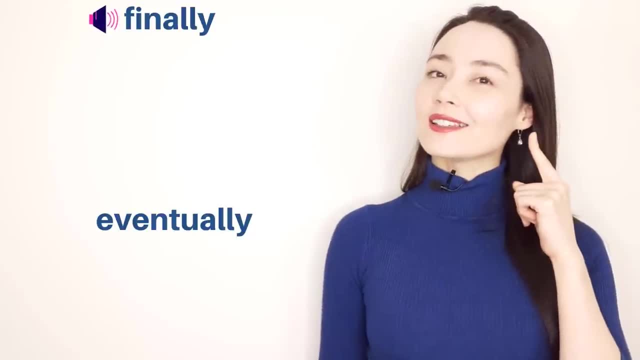 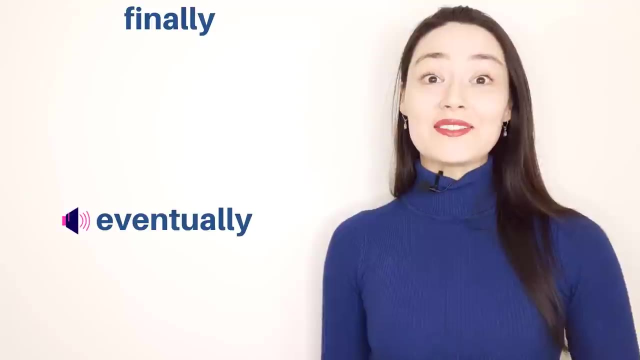 Jenna got married recently. They recently bought a house. These are one-time actions I cannot use lately. Phew, we're halfway there. Let's keep going with finally and eventually, Finally, finally- We don't say finally, Eventually, eventually. Finally, after waiting a long time for something. 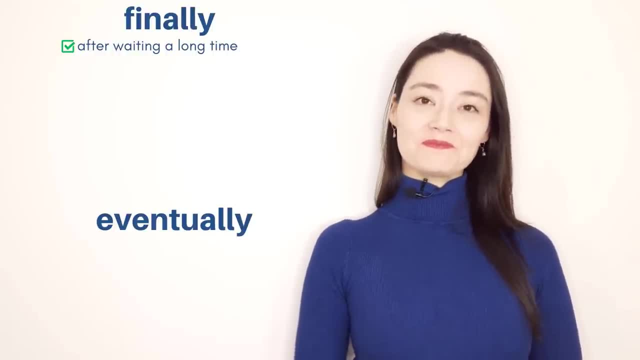 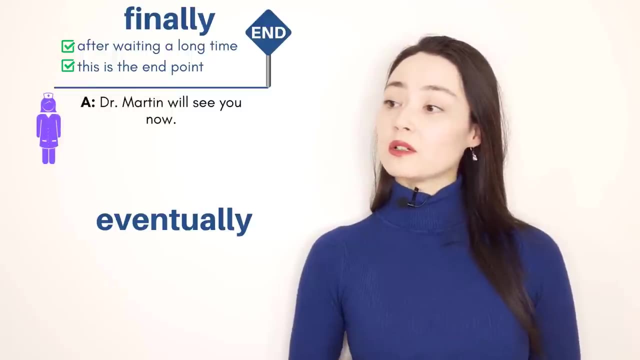 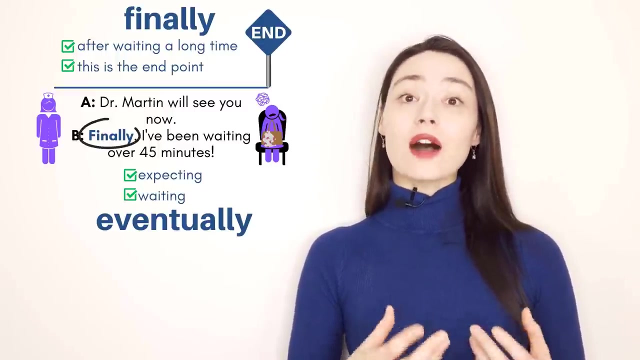 we are expecting. This is the end point. Dr Martin will see you now, Finally. I've been waiting over 45 minutes. Was I expecting appointment? Yes, Was I waiting a long time? Yes, And you can see I use the one word: finally, We. 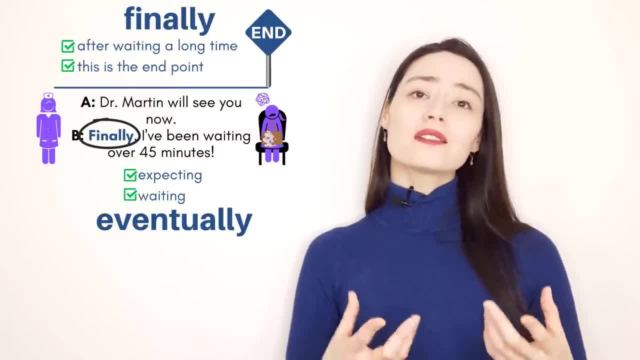 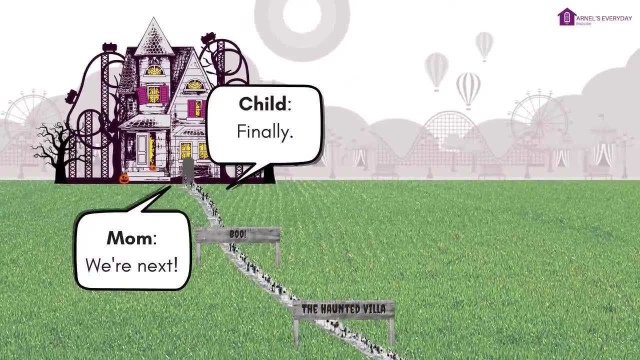 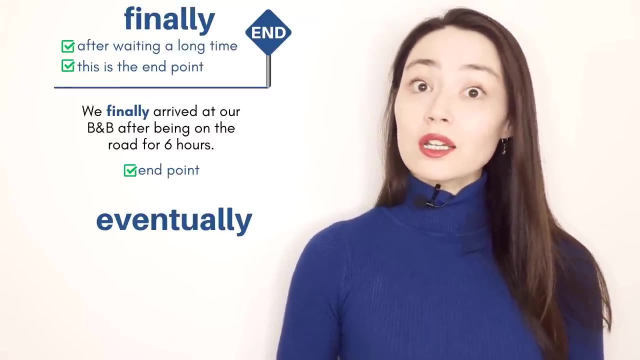 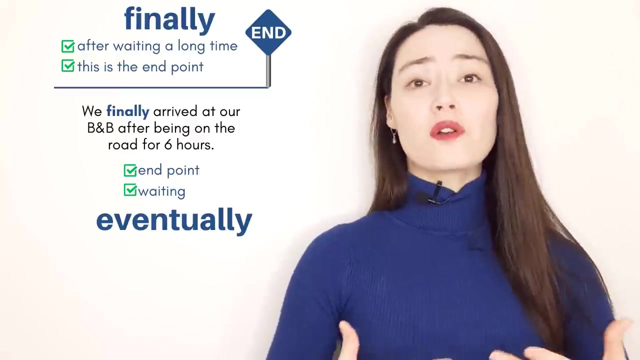 often use just that one word when we are happy: something happened, We're next. Finally, we finally arrived, arrived at our B&B after being on the road for six hours. Is this our end point? Yes, it's our destination. Were we waiting a long time? Yes, I mean being on the road. 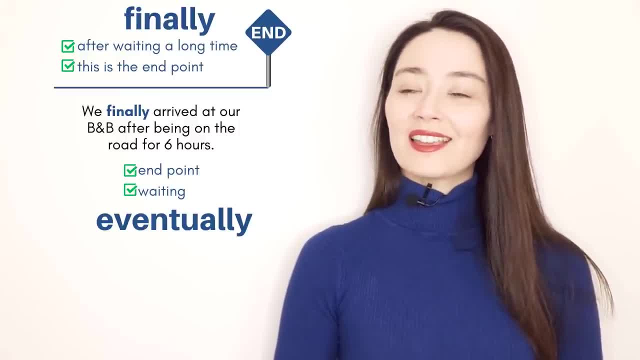 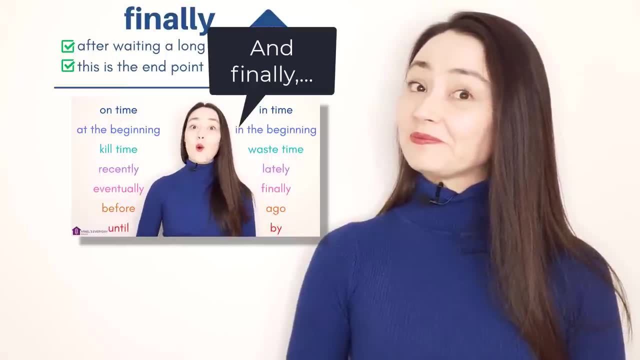 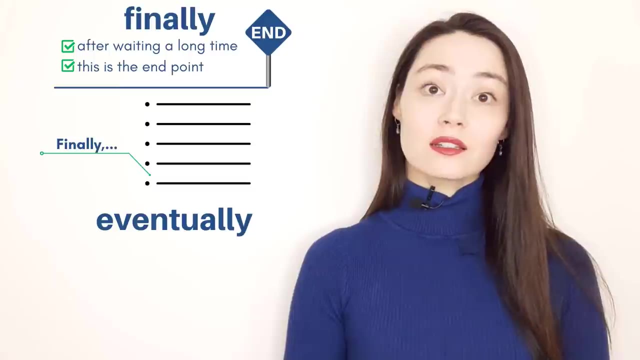 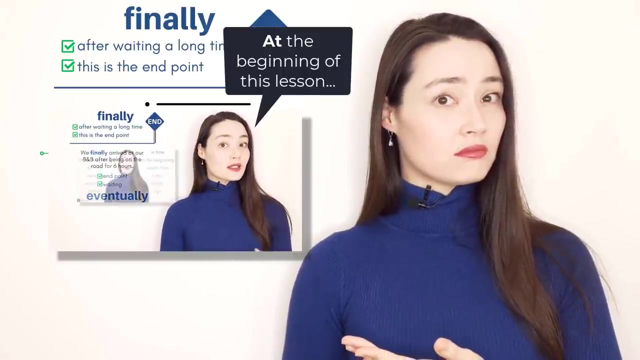 for six hours is a long time. And remember at the beginning of this lesson I said, and finally until or by, We also use finally to introduce the last thing in a list. And remember like ten seconds ago I said, and remember at the beginning of this lesson I said I used at the beginning because I really wanted to. 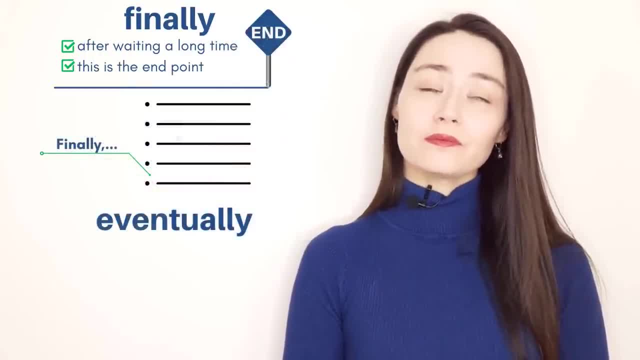 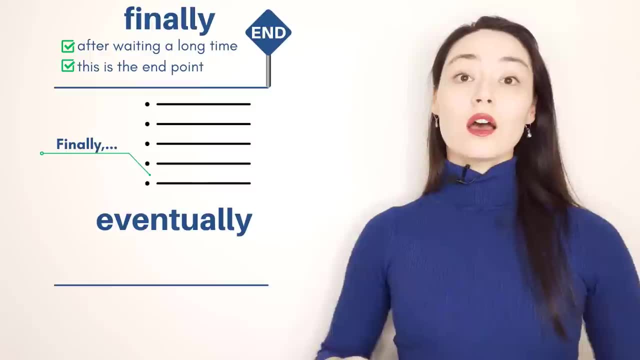 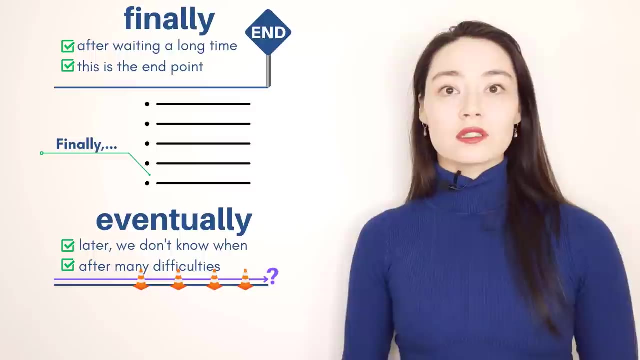 emphasize the start of this lesson And remember like three seconds ago I said- I'm joking, Let's keep going. Eventually, later- we don't know when- After many days difficulties, That feeling is really important with: eventually I'll never get a job. 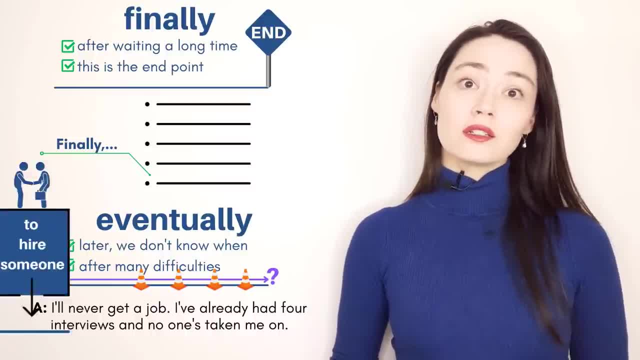 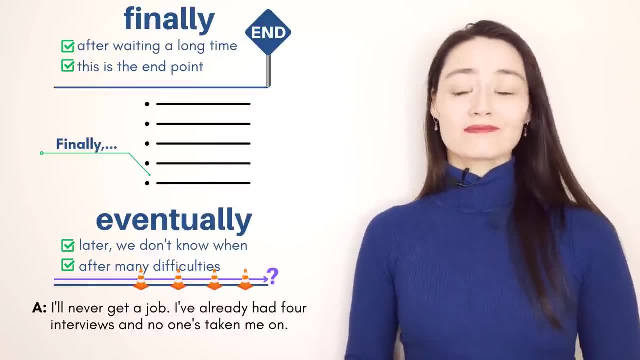 I've already had four interviews and no one's taken me on. If you take someone on, you hire them. No one's hired me, no one's taken me on. Just keep going. eventually you will find a job. Do we know when? No, Will there be many difficulties? Yes, finding a job is hard work. 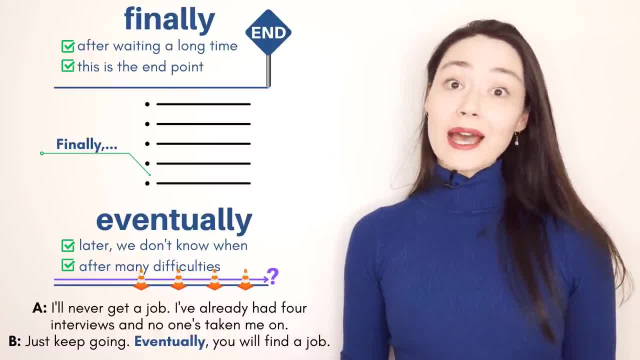 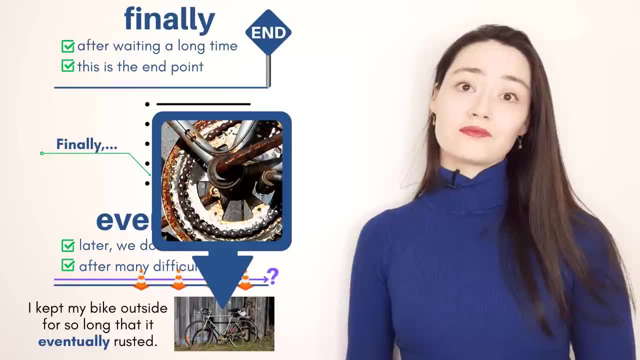 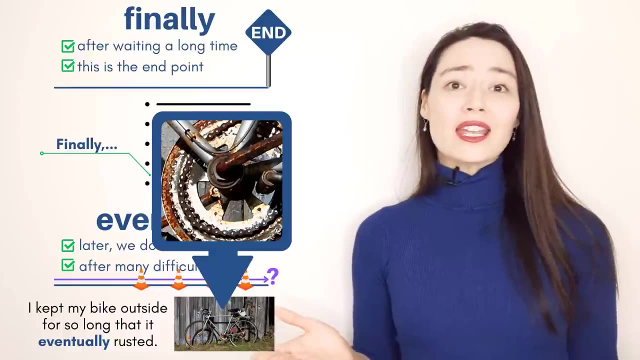 We don't only need to use a future tense, we can use a past tense. I kept my bike outside for so long that it eventually rusted. Did I know when? No, What's the difficulty here? Well, rain again and again and again is bad. 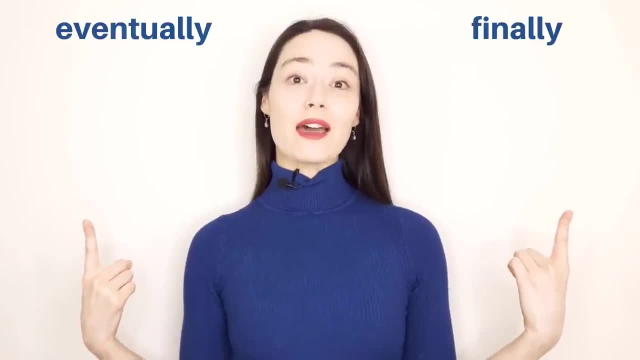 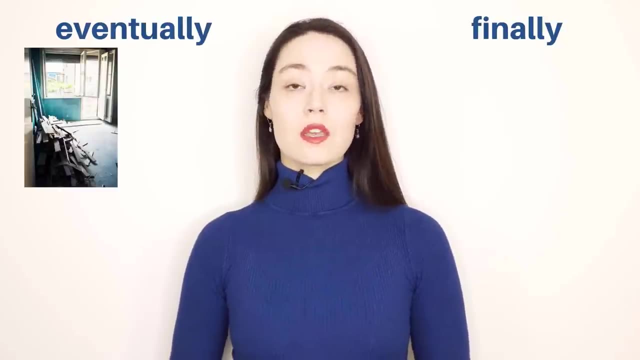 Bad for bikes. Let's compare these two adverbs. in the same situation, There's been a pile of wood sitting in my garage for months. My husband keeps saying he'll get rid of it. If we get rid of something, it means to remove something. 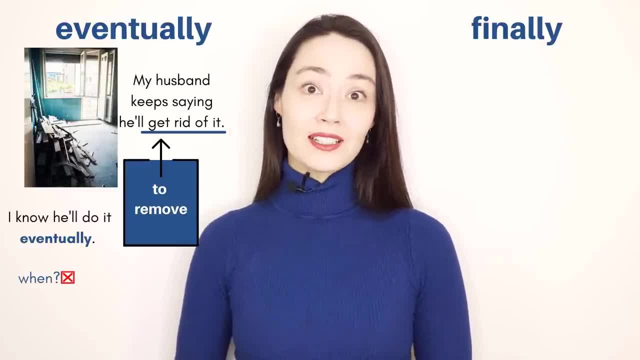 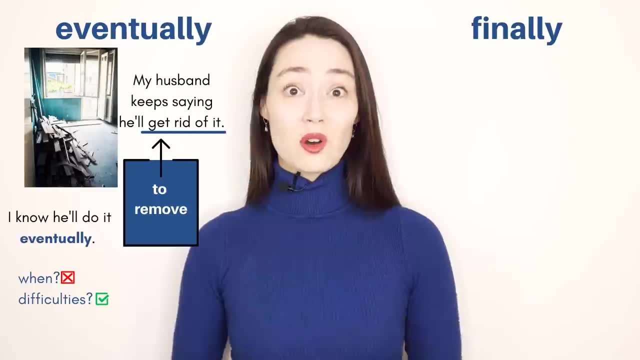 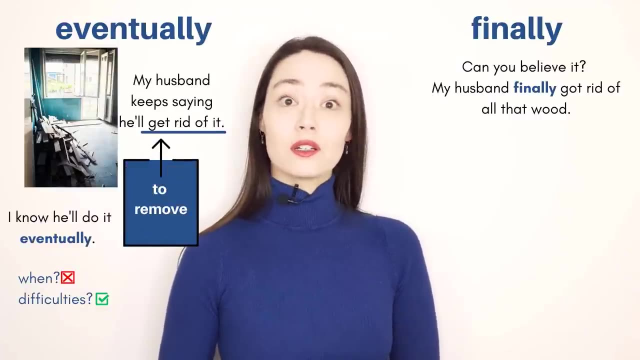 I know he'll do it eventually. Do I know when? No, Am I having difficulties? Yes, I'm annoyed. Can you believe it? My husband finally got rid of all that wood. Is this the end point? Yes, the wood is gone. Did I wait a long time? Yes, 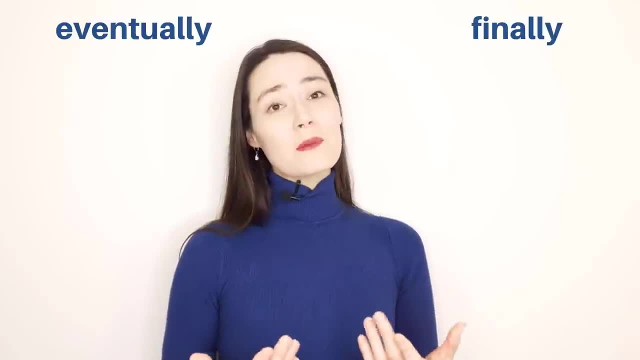 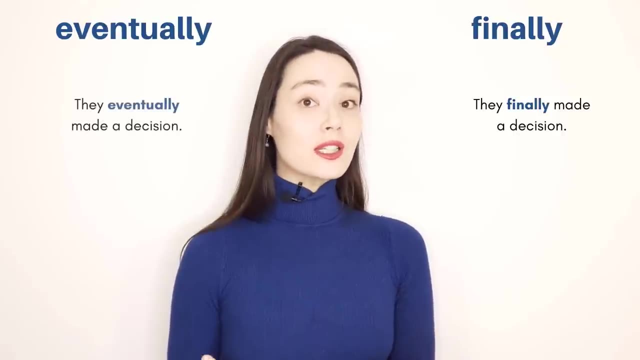 Okay, just like on time and in time. sometimes these two adverbs can be used interchangeably. For example, they finally made a decision. They eventually made a decision Here. these really mean the same thing. If you want to be really specific, I would say the person using finally. 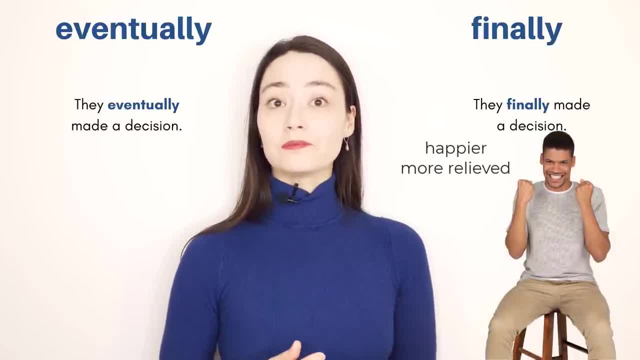 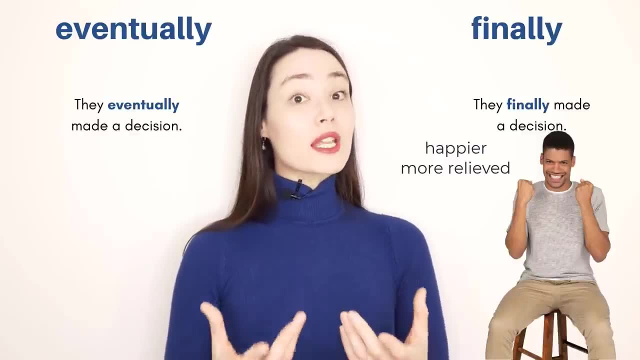 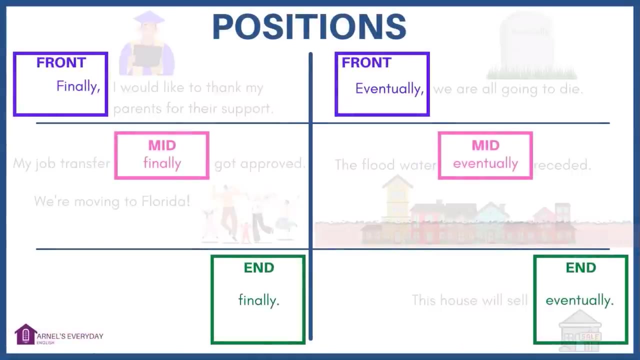 is happier and more relieved. In this lesson, I think these two adverbs are what students confuse the most, so let's do a few more examples. Let's look at those positions: Front position, mid position and position. Finally, I would like to thank my parents for their support. 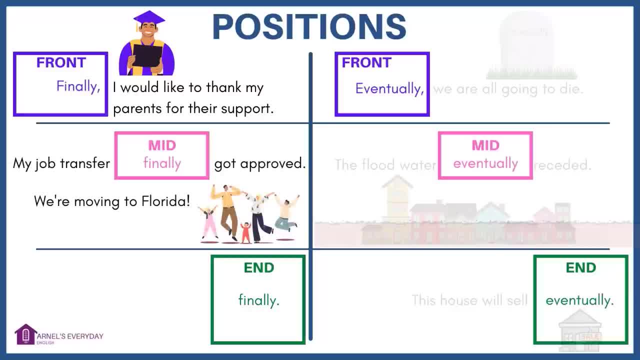 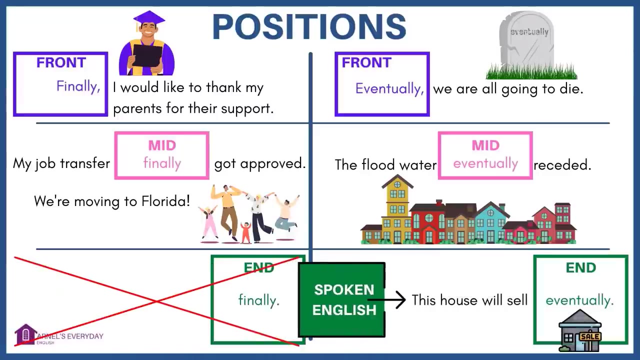 Mid position- My job transfer finally got approved. We're moving to Florida. And position No: Front position: Eventually we are all going to die. Mid position: The flood water eventually receded. End position, And normally this is only in spoken English. This house will sell. 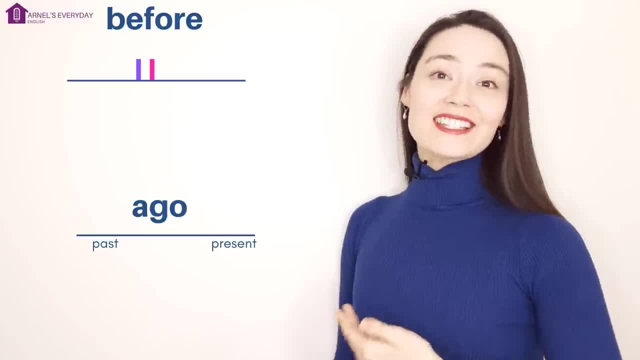 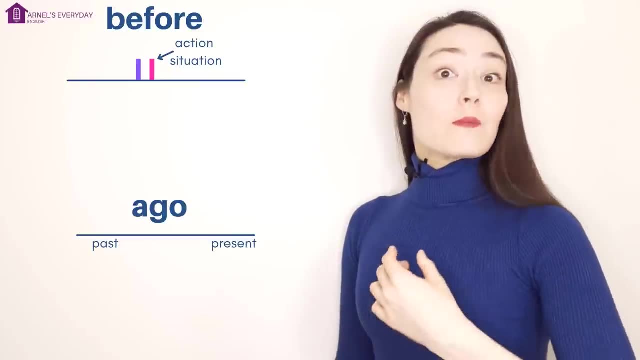 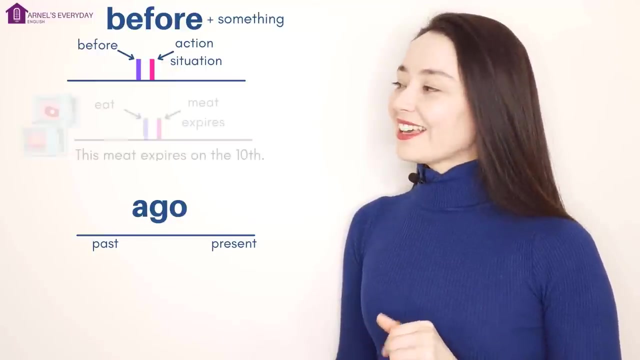 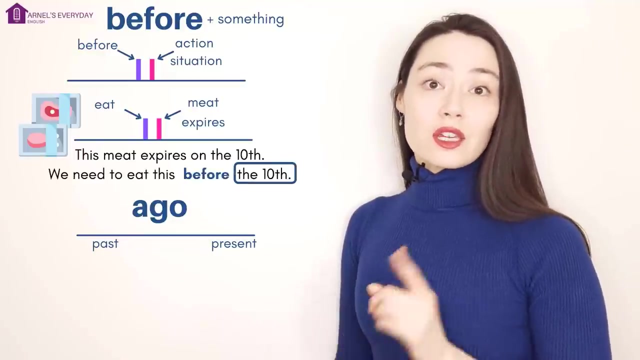 eventually. Okay, before and ago. Here I have something This could be an action or a situation. Before is always this time Before something. Imagine this meat expires on the 10th. We need to eat this before the 10th, just to be on the safe side. 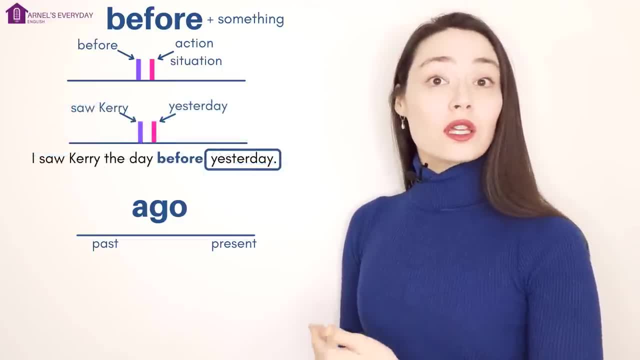 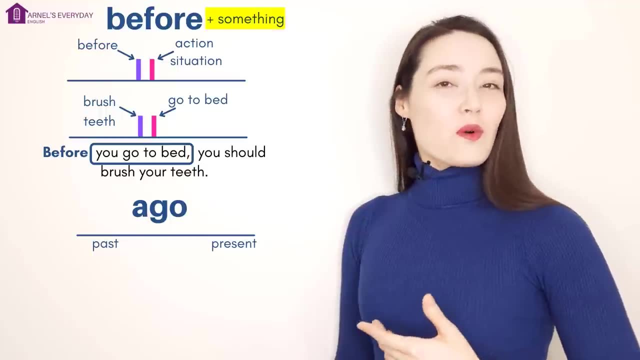 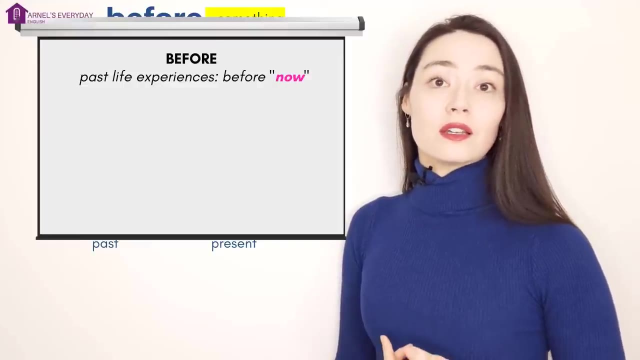 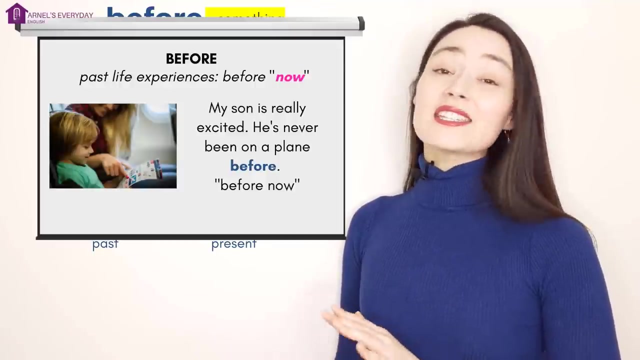 Yesterday. I saw Carrie the day before yesterday. Before you go to bed you should brush your teeth. So before, something is clear. But we often use before when we're speaking about past life experiences, because we mean before now. My son is really excited. He's never been on a plane before. 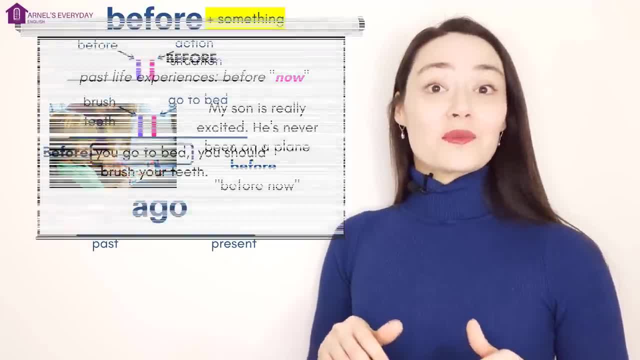 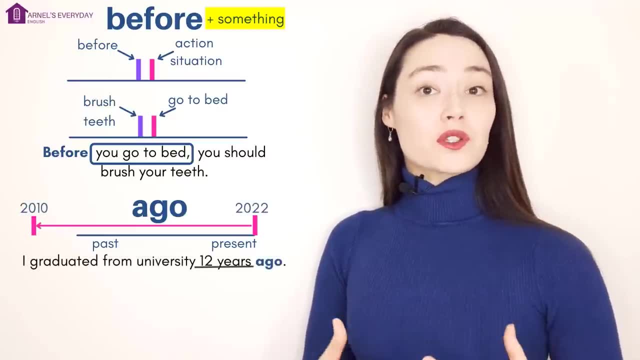 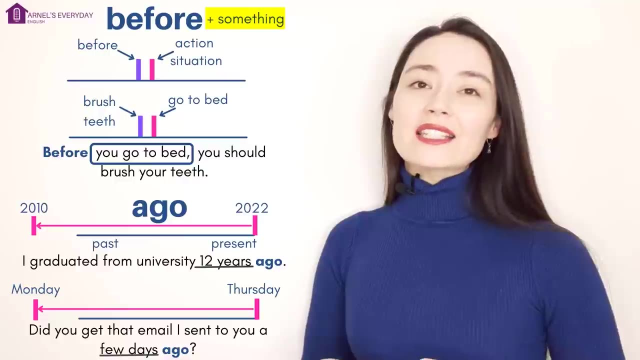 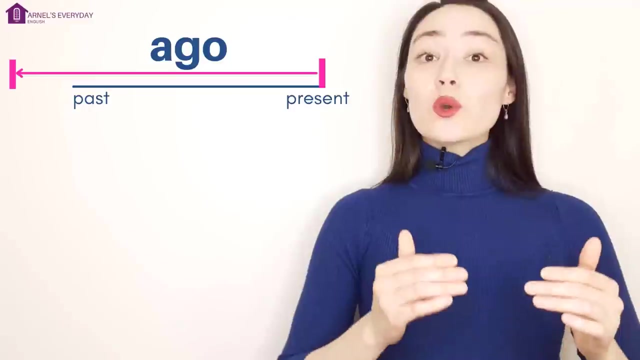 Before now, Ago From the present, From the present further into the past. I graduated from university 12 years ago. The time is clear. Did you get that email I sent to you a few days ago? If today's Thursday a few days ago would have been Monday, We know ago means from the present into the past. 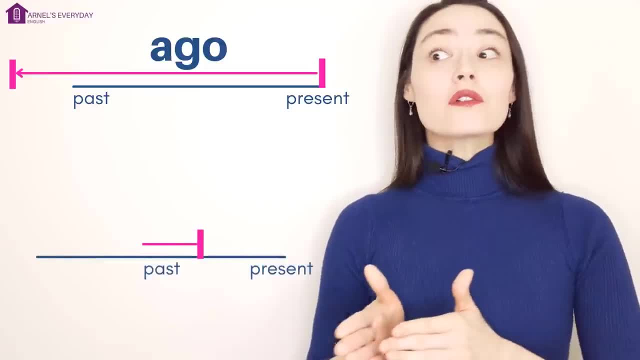 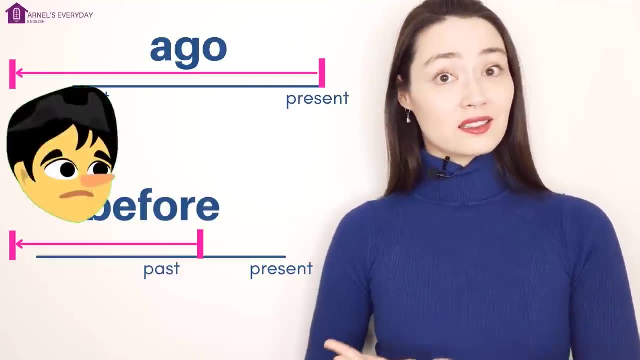 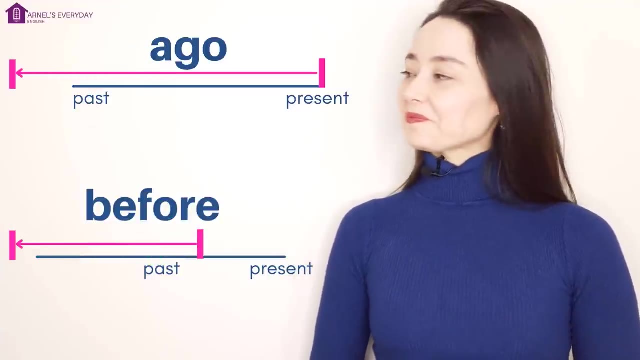 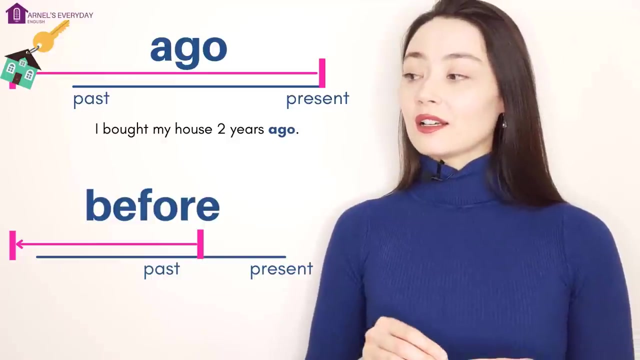 If we want to go from a past point further into the past, we need to use before. And you might be feeling like this. Let's do before. do an example: I bought a house two years ago. That's clear From the present Last. 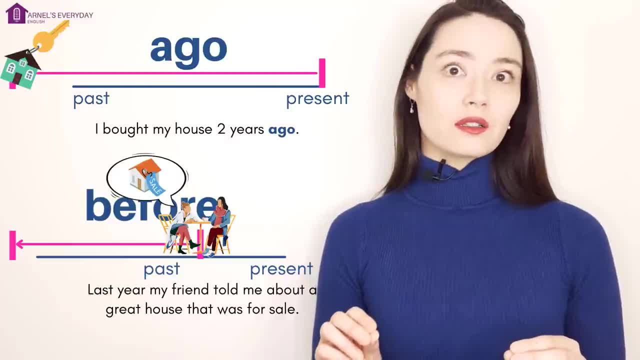 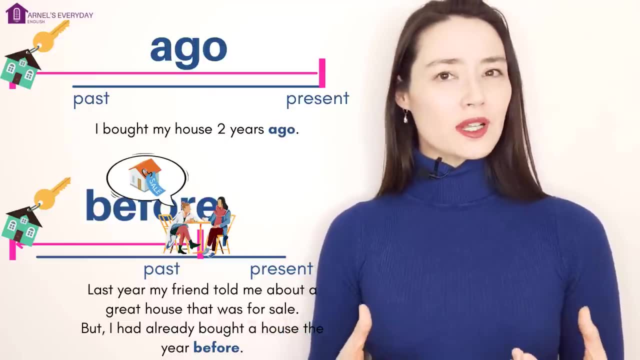 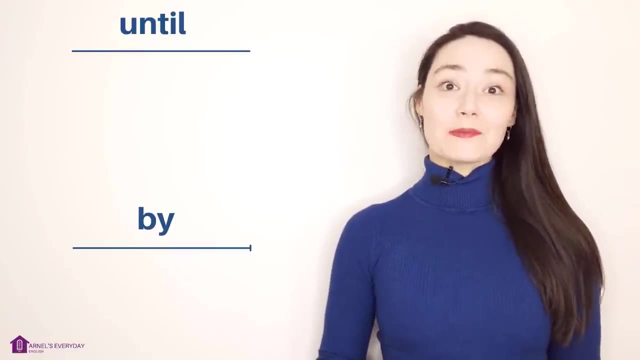 year my friend told me about a great house that was for sale, but I had already bought a house the year before. Can you see the points on my timelines? Last pair, before the test, Until and by, I know there's been a lot of lines- lesson 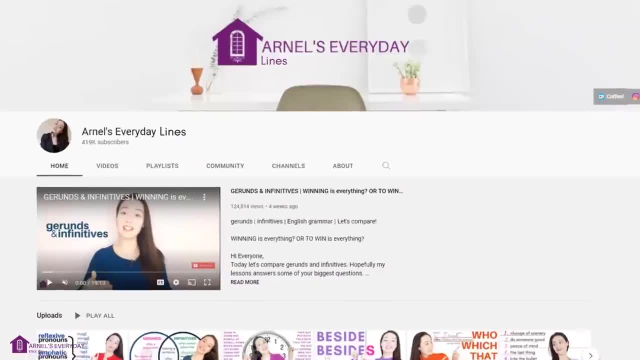 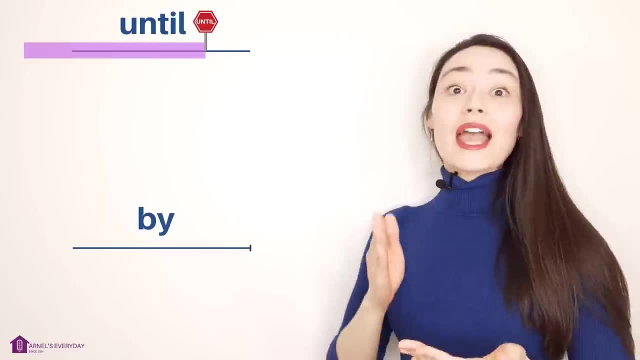 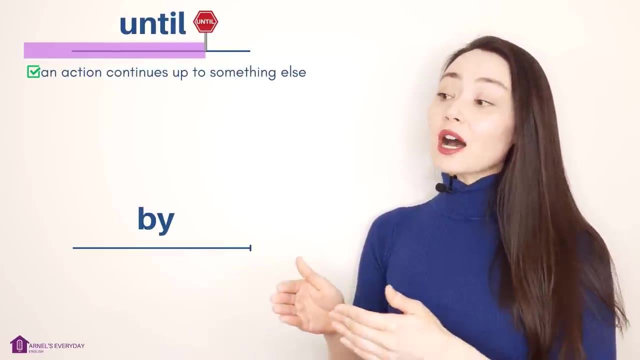 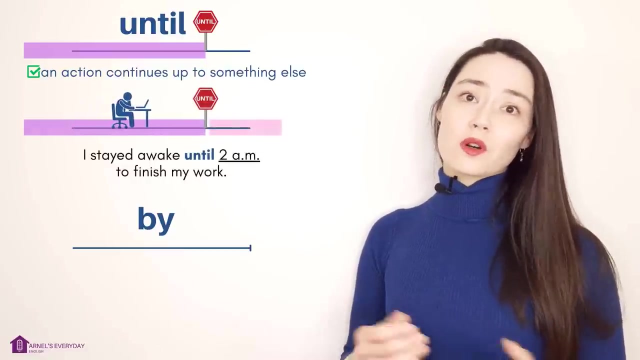 I like lines. I should change my channel name to Arnel's Everyday Lines. Okay With until an action continues and then stops. Until is your stop sign. So an action continues up to something else. I stayed awake until 2 am to finish my work Here. it's clear I was awake and 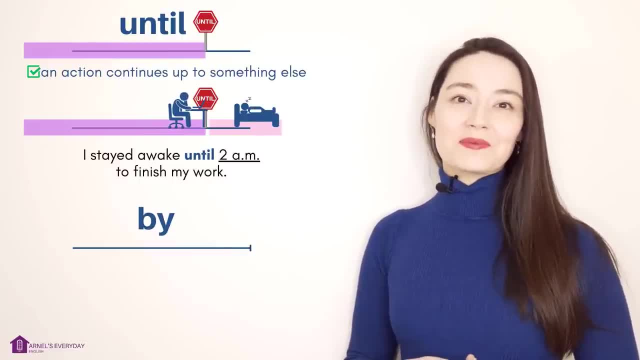 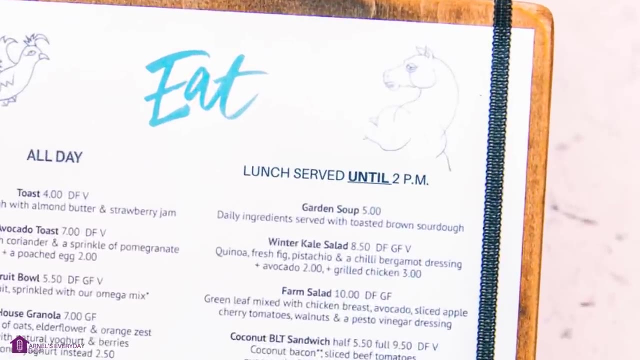 after 2 am I was sleeping. My parents are staying with me until Monday. They leave Monday afternoon. Or if you go to a restaurant, maybe you see this on a menu: Lunch served until 2 pm. Here it's clear at 2 pm the lunch service stops. 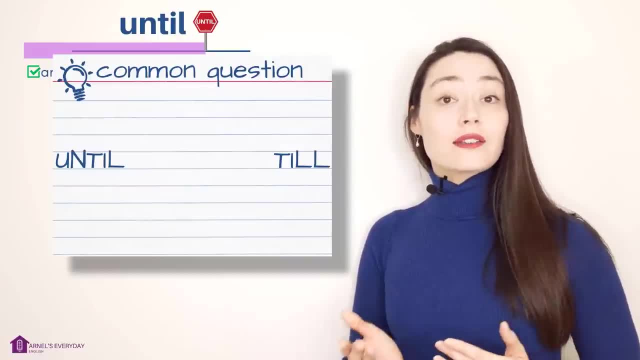 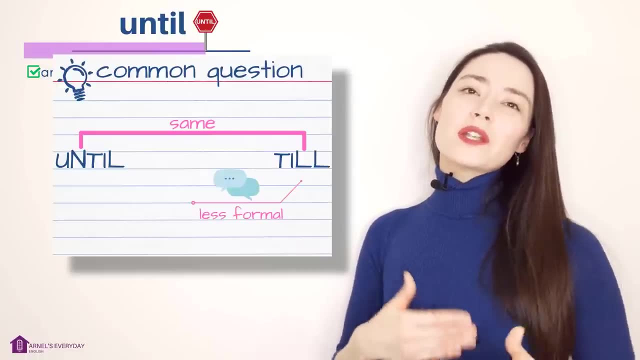 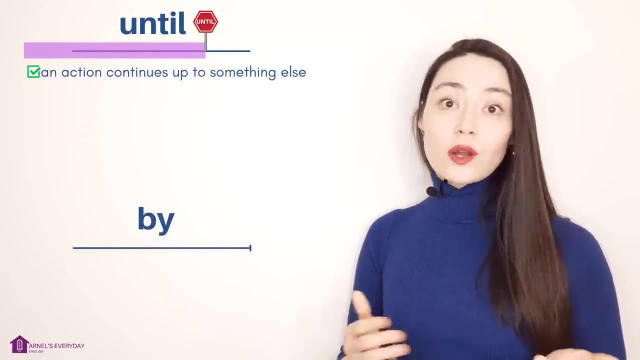 Common question: What's the difference between until and til? They mean the same thing. I would say till is more common in spoken English and less formal than until. Until can also be followed by a clause, Not just one word. Mom, can I get? 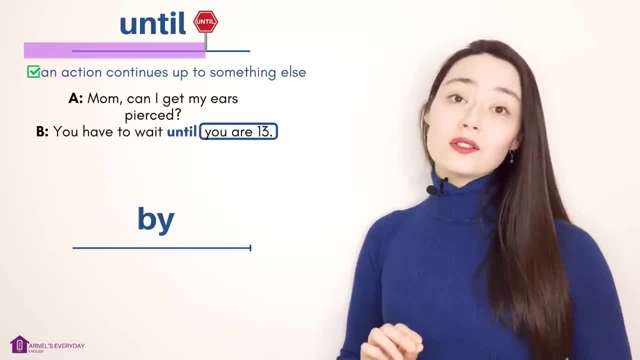 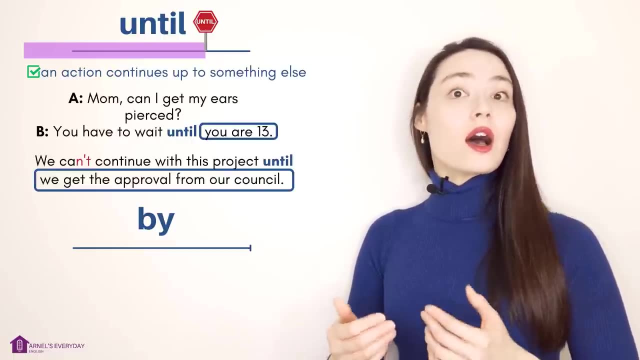 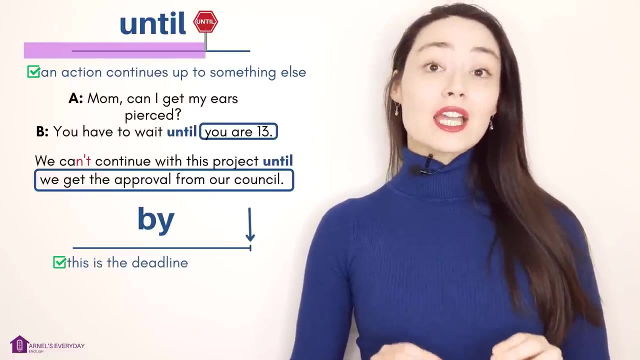 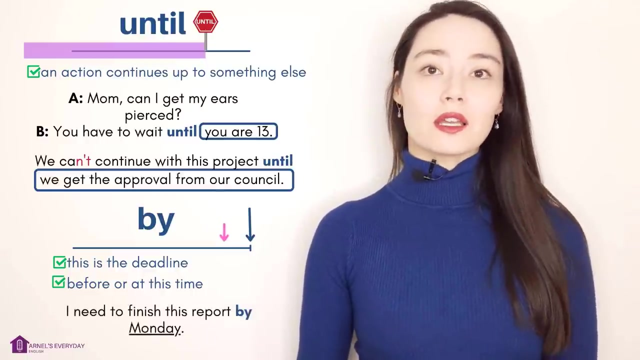 my ears pierced. You have to wait until you are 13.. At 13 the waiting stops. We can't continue with this project until we get the approval from our council By This is the deadline. An action has to happen before or at this time. I need to finish this report by Monday. Monday is. 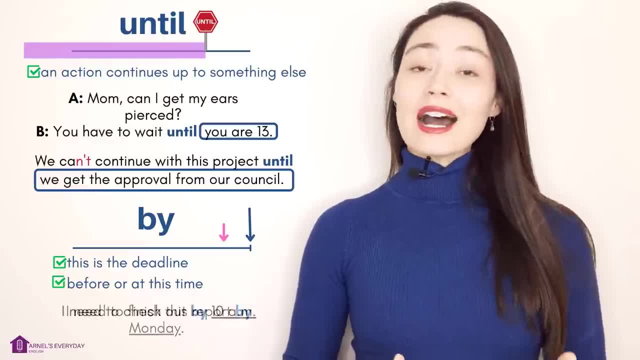 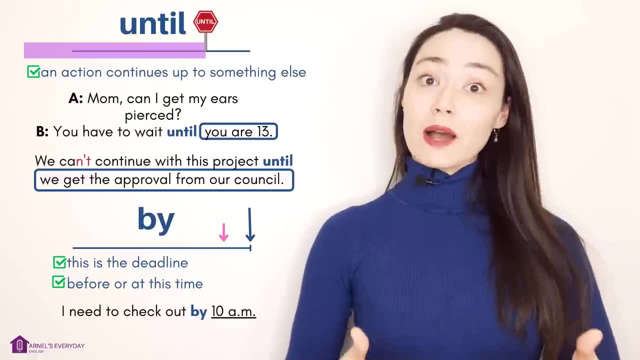 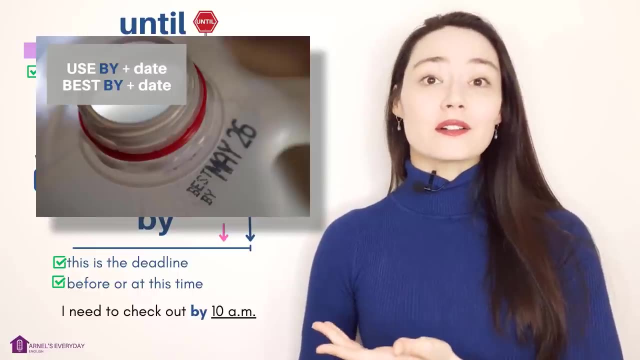 my deadline. If I'm staying in a hotel, I need to check out by 10 am. 10 am is my deadline. On food packaging. you might see this: Use by plus date, Best by plus date, Kind of like on this milk carton here. You want to drink this milk by. 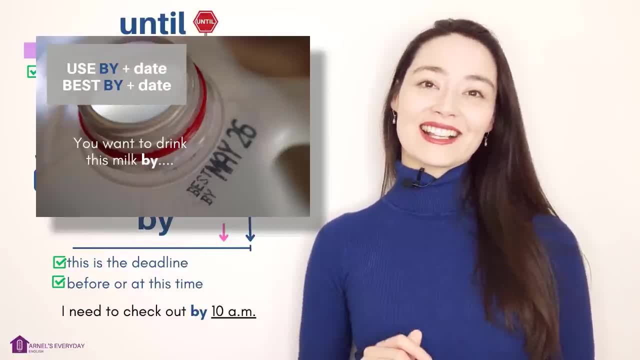 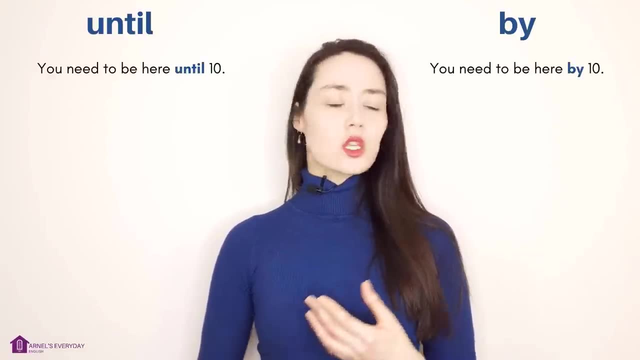 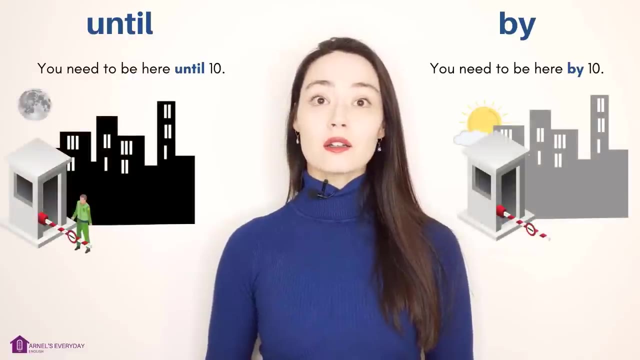 What's the date on this? May 26.. Let's compare again. You need to be here until 10 am. You need to be here by 10 am. There's a big difference. Let's say we're speaking about a security guard. He's working the night shift. He needs to work. 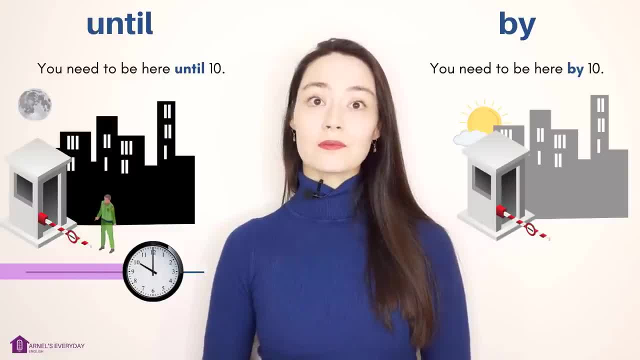 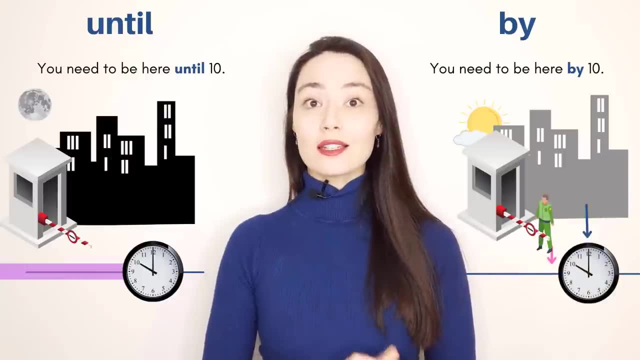 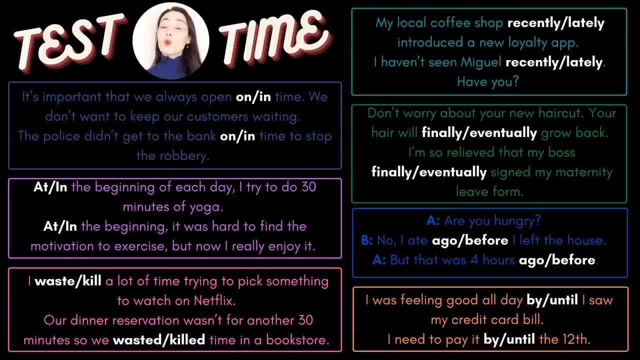 until 10 am. He can leave at 10 am. You need to be here by 10 am. Here, it's clear. he needs to start work at 10 am. Are you ready for a test? Let's take a look. Okay, what I'd like you to do is to select. 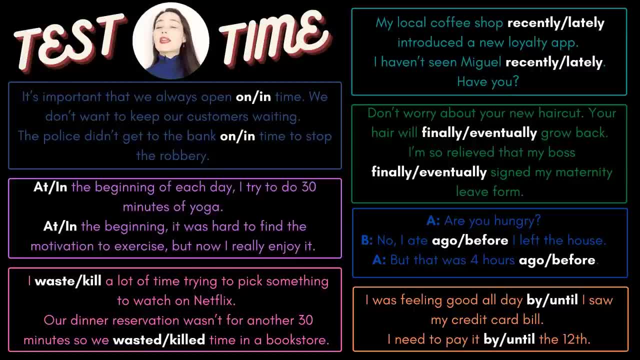 the right option. There can be more than one option possible, and don't just look at the one word. Look at the grammar surrounding the options. Pause the video to do this. Here are the answers. Don't forget to let me know how you did in the comments below. 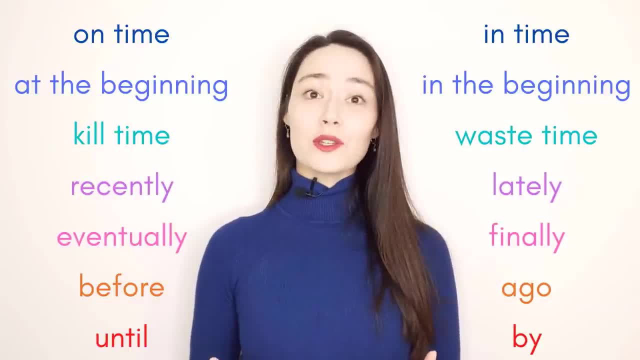 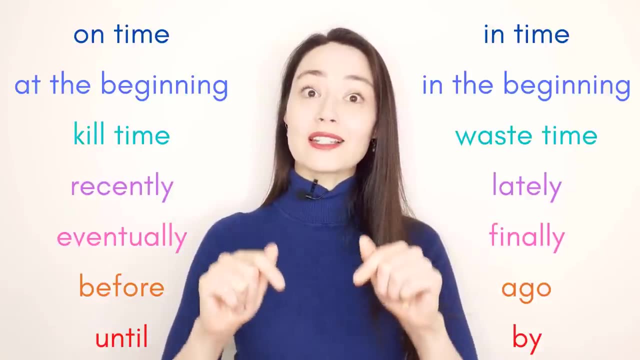 Wow, I really enjoyed making this lesson for you. Thank you so much for watching. I hope this lesson was helpful. I'll see you next time. Don't forget to let me know your test results down below. Thank you very much, Bye.